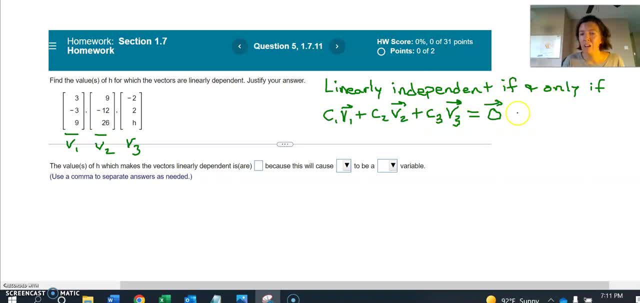 independent if, and only if, this equation has only the trivial solution. So let me finish writing out this: It's linearly independent if, and only if, this equation has only the trivial solution. Which think of it as the cheap way to solve this equation, which is just to multiply every one of those vectors by zero. 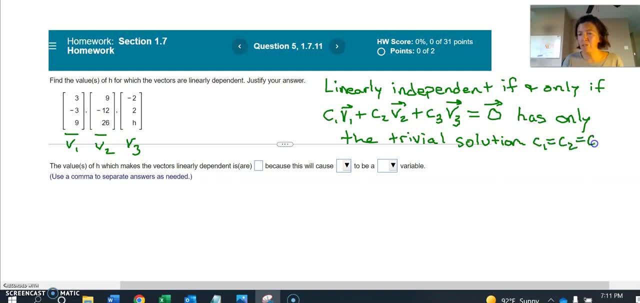 So c1 is zero, c2 is zero, c3 is zero. All the scalars are zero. You just multiply zero times every vector and voila, I've got the zero vector. Well, that's not really an interesting way to solve that equation. 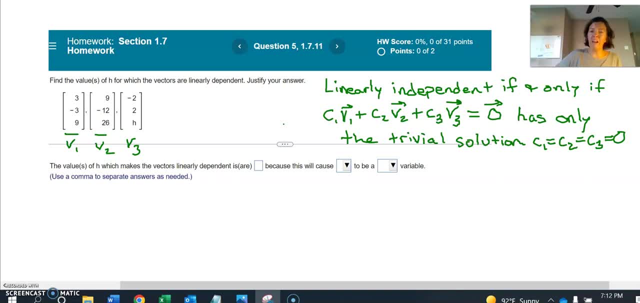 So what we're really more interested in is what's called non-trivial solutions, where at least one of these coefficients- c1,, c2,, c3, is not zero. Now I was going to paraphrase, but I ended up writing out the full definition, so I might as well clarify the beginning here. 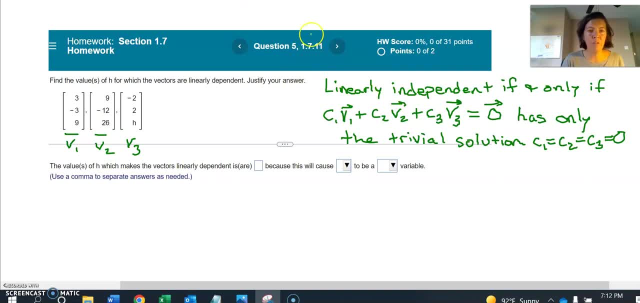 So I need to say, well, what's linearly independent? So this is the definition of the collection of vectors v1, v2, v3 being linearly independent. If we take a linear combination of those vectors equal to the zero vector, and we learn that, well, the only way to accomplish this is to make every scalar zero, then they're linearly independent. 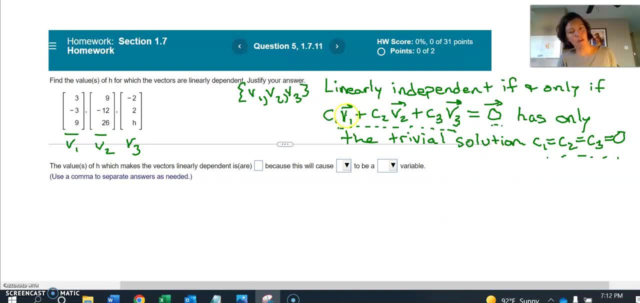 If we can find an interesting way of solving that, like: 2 times vector 1 plus 3 times vector 2 minus vector 3 equals zero, well then those are linearly dependent. Okay, so the task here is to find the value of h for which the vectors are linearly dependent. 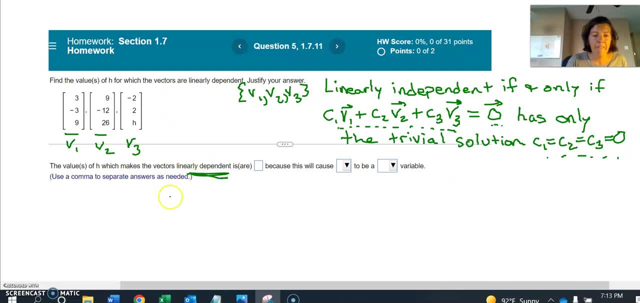 So we will. So we want this system to have a non-trivial solution, And I believe it was mentioned in this section, or no, probably previous section, that a homogeneous system has a non-trivial solution if, and only if, there are free variables. 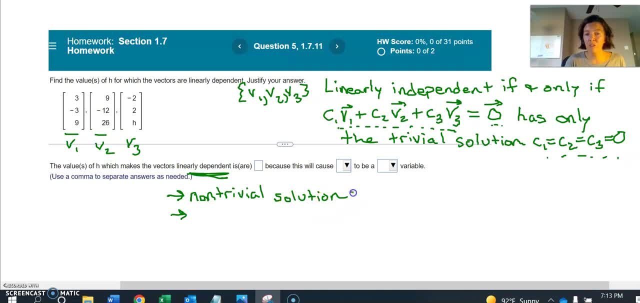 So that homogeneous equation is going to have non-trivial solutions, plural: if you have one of them, then you're always going to actually have infinitely many if there are free variables, at least one free variable. Okay, let me see if I can scroll down here. 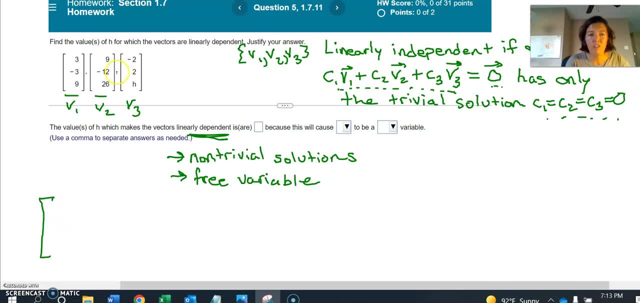 So suppose we work on solving this equation where v1, v2, v3- are these guys here? Well then, that equation could be represented as an augmented matrix where column 1 is that first vector, Column 2 is the second vector. 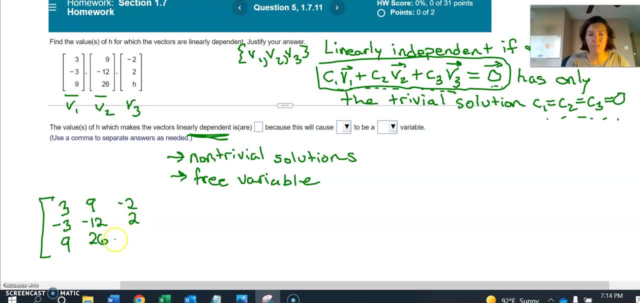 Column 3. And I believe that was discussed in one of your last two sections- how this vector equation can be represented Using this augmented matrix. Okay, So now we want to solve the system, So I want to reduce this thing. Now. there was some discussion, also in GroupMe, about how the pivots don't have to be ones. 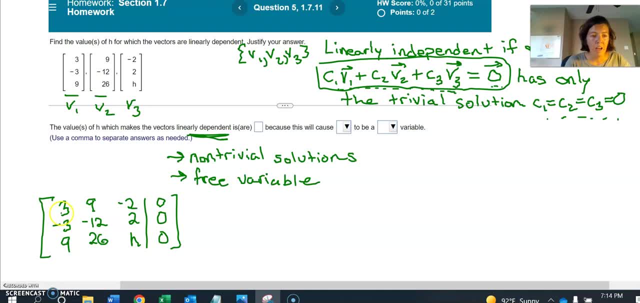 And they don't. If we're looking for echelon form, they don't have to be ones And notice. we're just trying to find conditions under which this is linearly dependent. We're not trying to find the actual solution set to the system. 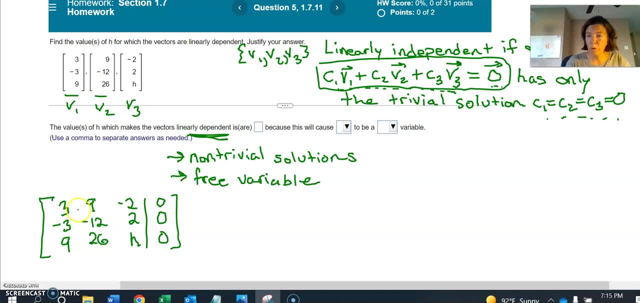 Okay, So we don't. We don't necessarily need to reduce this all the way to reduced echelon form. We could just stop with echelon form. So, anyway, pivots don't have to be ones. They don't. And in fact I mean these entries below that 3, they're both multiples of 3.. 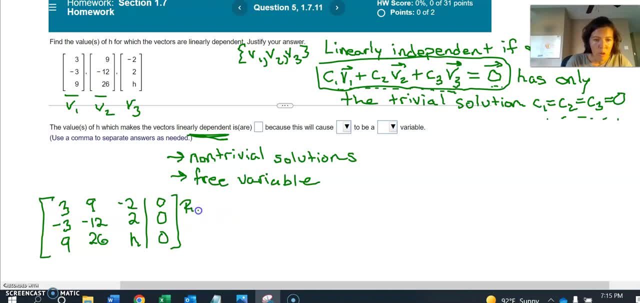 So I might as well just leave it as a 3.. We can do row 1 plus row 2. That'll give us a 0 in this position here, So I'm going to leave row 1 alone. Row 1 plus row 2 gives me 3 plus negative 3.. 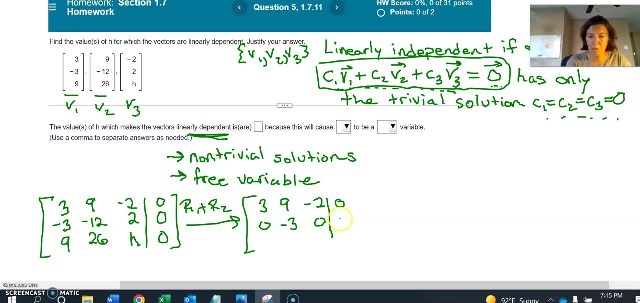 So that's 0.. 9 plus negative 12.. Negative 2 plus 2.. 0 plus 0.. I'm going to also do negative 3 times row 1 plus row 3 in order to. So if I do negative 3 times 3, I get negative 9.. 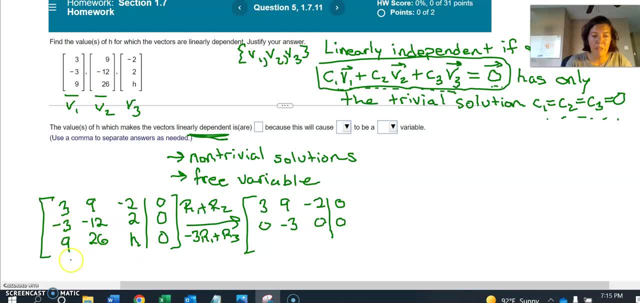 That'll clear out this 9 here. So that'll give me negative 9 plus 9.. And negative 27 plus 26.. So negative 1. And then negative 3 times. this would be positive 6 plus h. I'm going to write it as h plus 6.. 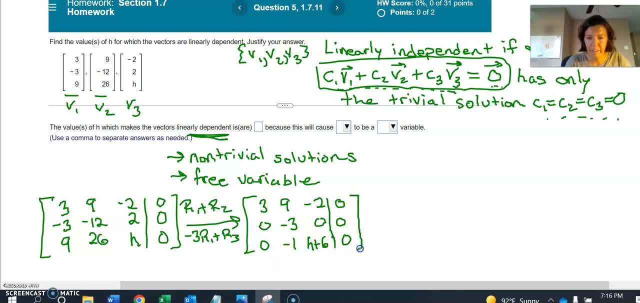 Okay, And then 0 plus 1.. I guess what I would do now, I mean. so this is a matter of personal preference- I suppose I'm going to swap these two rows. So swap row 2 and row 3.. 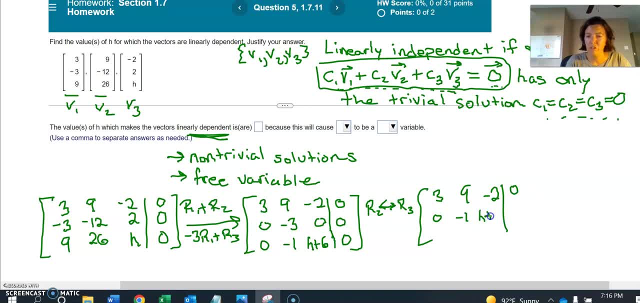 So this is 0, negative 1, h plus 6. And then 0, negative 3,, 0, 0 here And then, Sorry about that, I should have muted my phone, Then I can do. I want to clear out this negative 3 here. 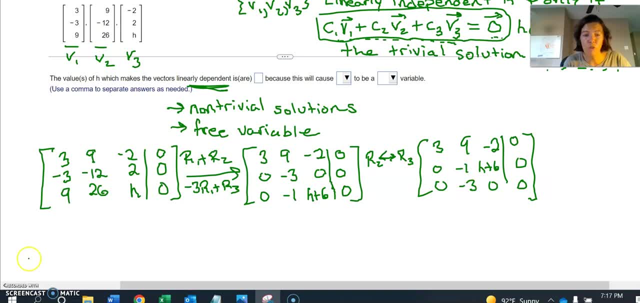 So I could do negative 3 times row 2.. Negative 3 times row 2.. Add that to row 3.. And then here I'm going to write out the arithmetic. Let me change colors. So if you, When you have variables in your 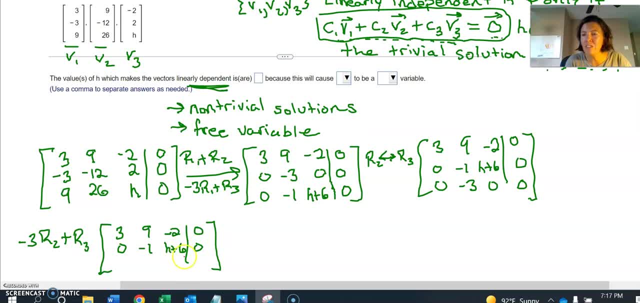 Well, not variables. If you have unknown values in your entries here, then you might want to write out your row operations the long way, The way I showed you guys in the notes, which is how I'm going to show it here. So, one step at a time, 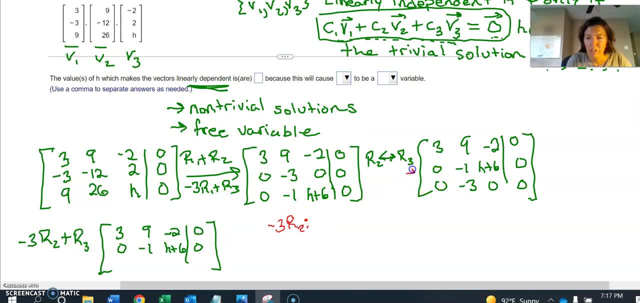 Negative 3 times row 2.. Here's my row 2. So negative 3 times everything, Everything. there would be 0,, positive 3. And then we have negative 3 times h plus 6. So that'll be negative 3h minus 18.. 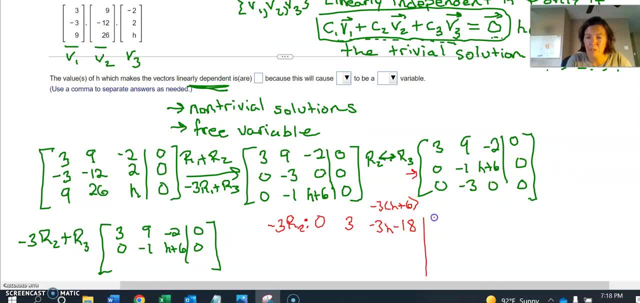 Right And then negative 3 times 0.. We're going to add that to what used to be in row 3, which was this: So 0, negative 3, 0, 0.. So the new row 3 is this: 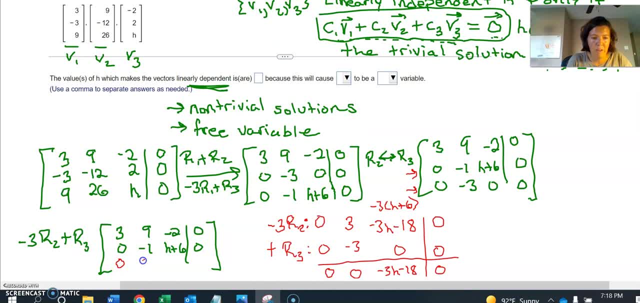 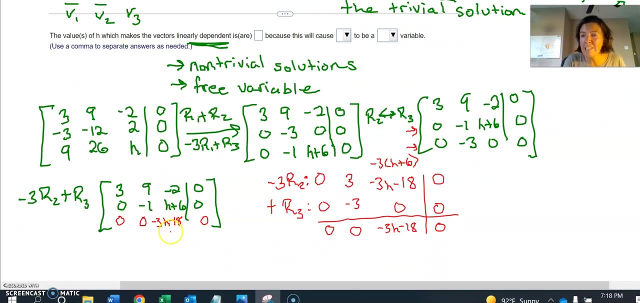 So I'm going to put that here: 0, 0, negative 3h minus 18.. Sorry about that. 0.. Okay, Now we can talk about solution sets. So we want this thing to have non-trivial solutions. 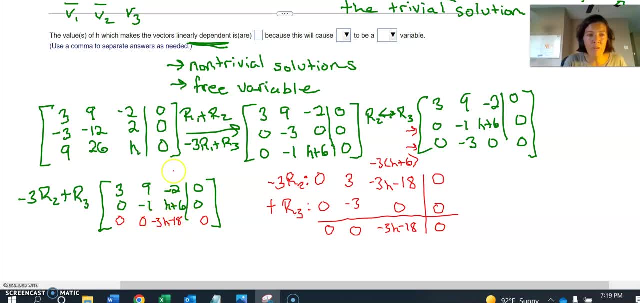 If this entry, right here, is anything other than 0, then like, say, this ends up being negative 16.. Then you're going to have negative 16 times x3.. Sorry, our unknown 0, c3.. This is c3. 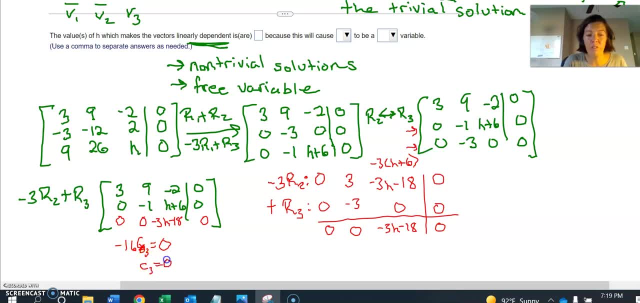 Divide both sides by negative 16. You get c3 equals 0. And then the dominoes fall. When you do back substitution, you're going to find out: well, then c2 equals 0, and then c1 equals 0,. 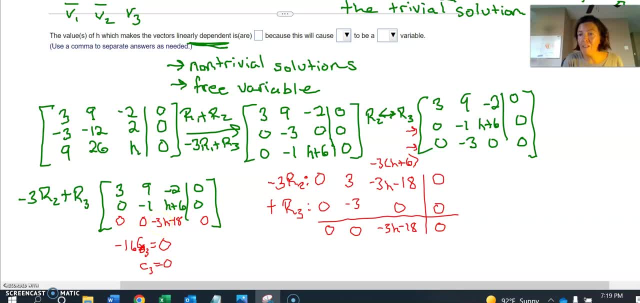 and you have only the trivial solution. When you have a pivot in every column, you end up with only the trivial solution with these homogeneous systems. So we don't want that to happen. We want this to be independent, So we need to have a free variable. 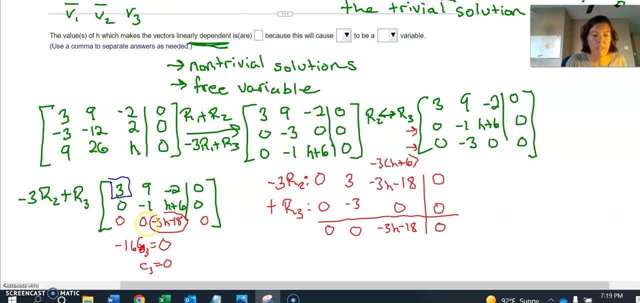 Notice that there's already a pivot in column 1. right here, There's already a pivot in column 2.. Depending on the value of h, there is potentially a pivot in column 3.. The only way we can avoid this guy being a pivot. 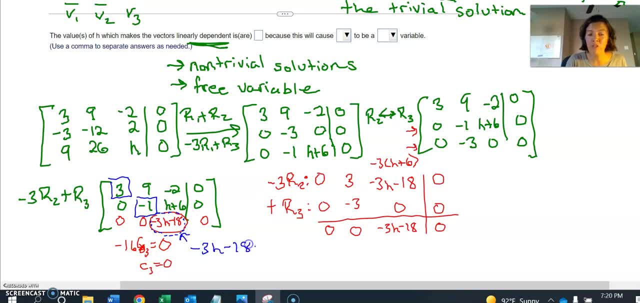 is if it's equal to 0.. Pivots, by definition, are the first non-zero entry in each row. So if this is 0, then there's no pivot in row 3, which means there's no pivot in column 3.. 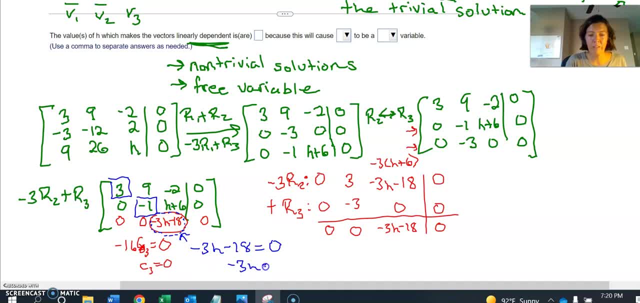 So if you solve this thing well, we can write that out. Let's see: move the 18 over divide by negative 3, we get h equals negative 6.. Yes, So if h is equal to negative 6,. 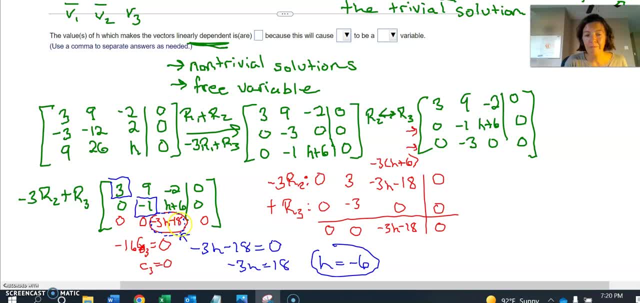 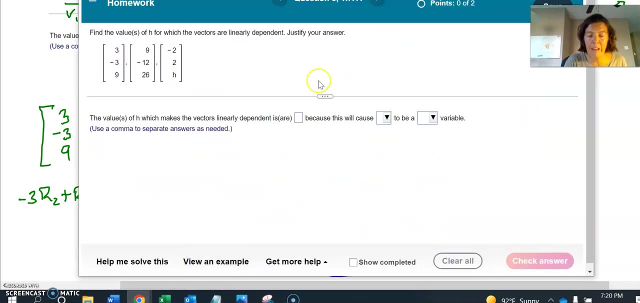 then this thing: this entry right here is 0.. We have no pivot in column 3.. x3 is a free variable. Okay, so I wanted to switch over. Before I end this video, I'm going to switch to my math lab. 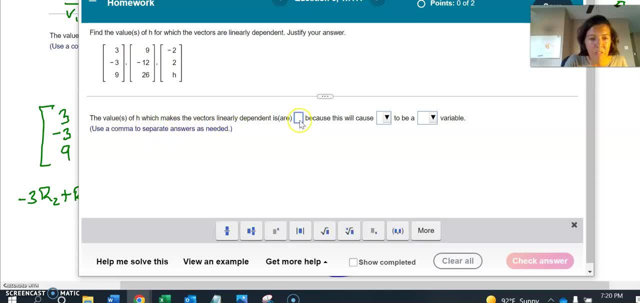 So the value of h, which makes the vectors linearly dependent, is negative 6, because then you'll have no pivot in column 3, so it'll cause x3 to be a free variable. Now x3, in the equation I wrote it's c3,.